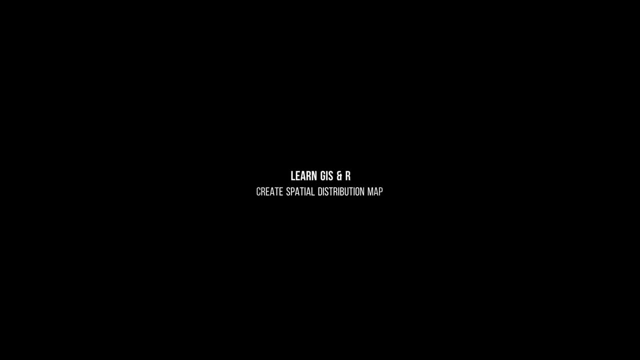 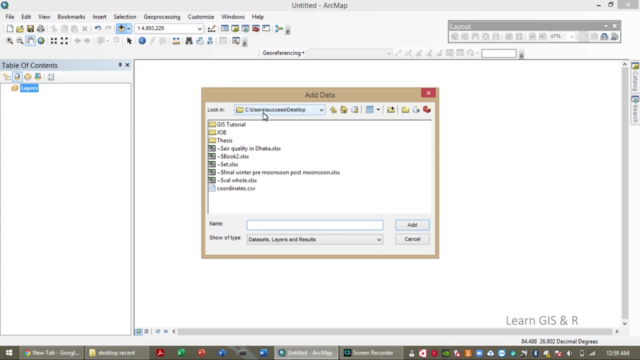 Today I'm going to show you how to create spatial distribution map using interpolation techniques. First, you have to import shapefiles of your desired location. If you don't have the folder connection, you can use this icon to connect your folder. Now I'm going to import my shapefile. 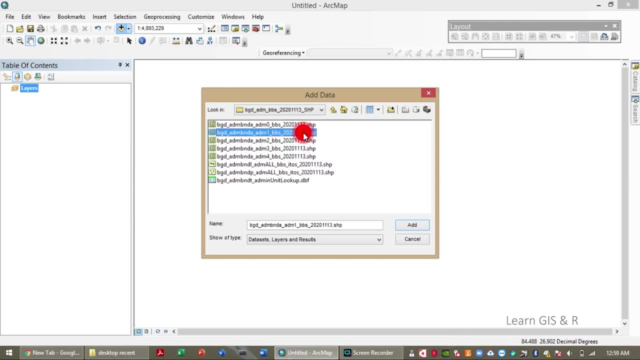 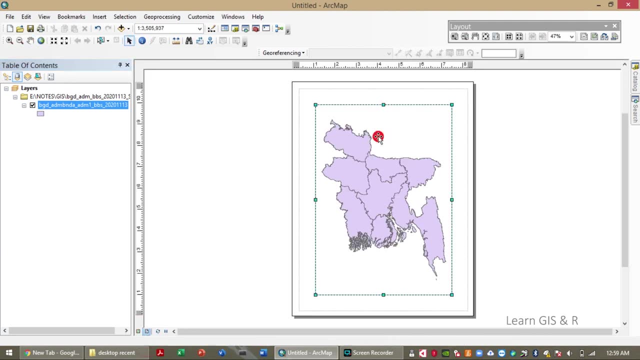 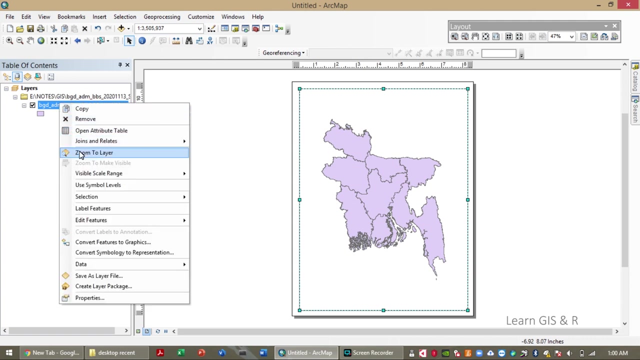 Yes, the shapefile has been imported. Interpolation actually predicts values for cells in a raster from a limited number of sample data points. It can be used to predict unknown values for any geographic point, data such as elevation, rainfall, chemical concentration or noise levels, etc. 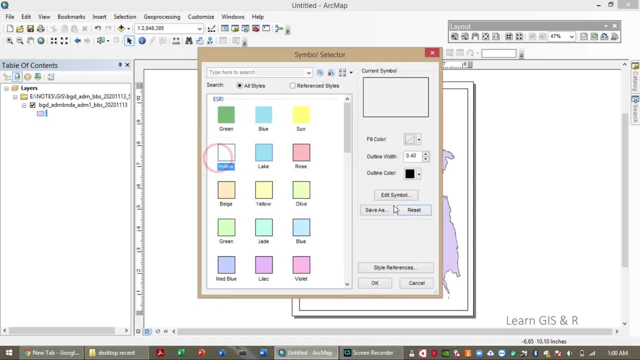 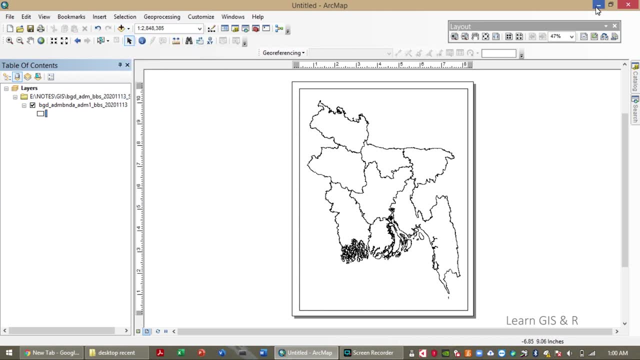 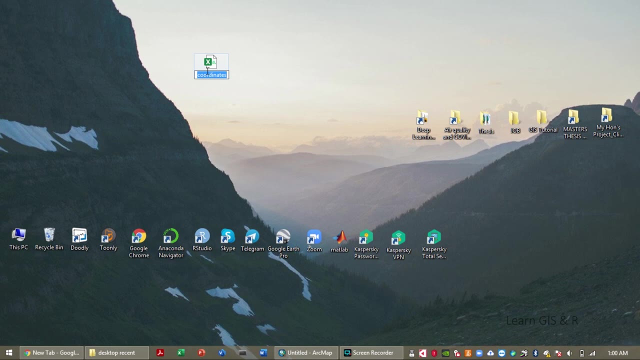 You can use any kind of data by using this map. Now I'm going to show you the data which I'm going to use in this tutorial, because you have to know how to arrange or how to prepare your data for this analysis. I have the data of: 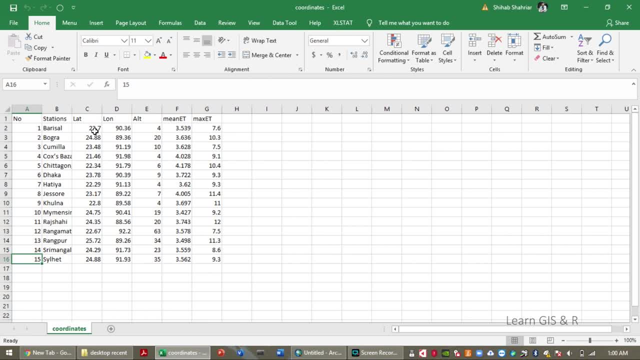 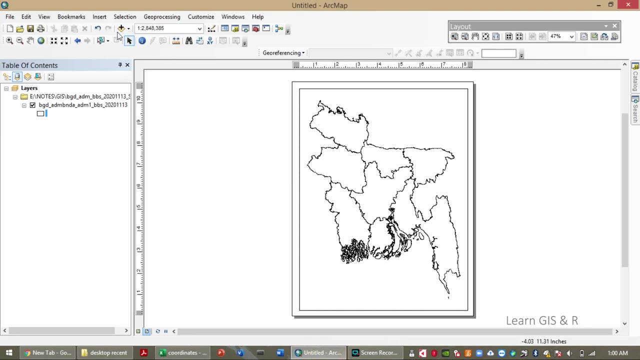 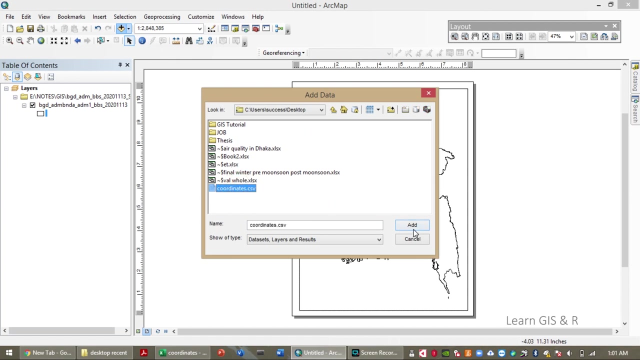 my country. If I put transpiration for my country for 15 stations with their coordinates, I mean the longitudes and latitudes. You have to arrange this data by this format. Now I'm going to import my data points here. Yes, the points has. 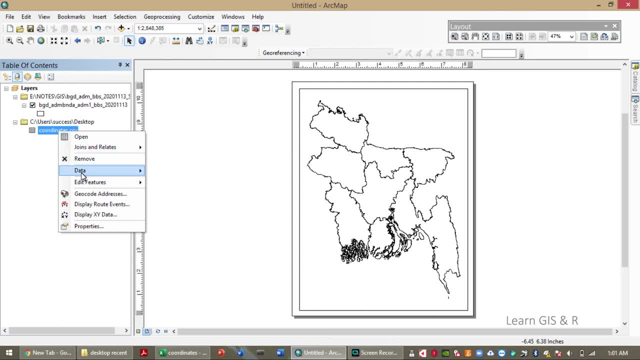 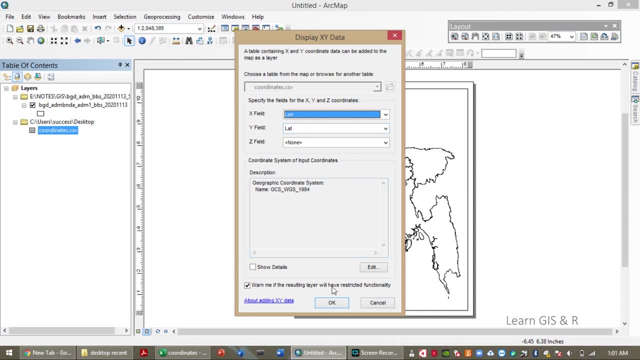 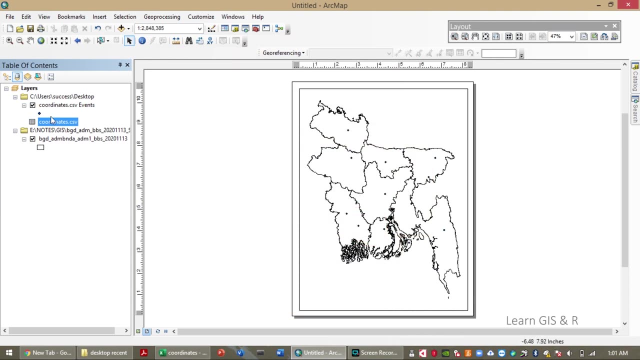 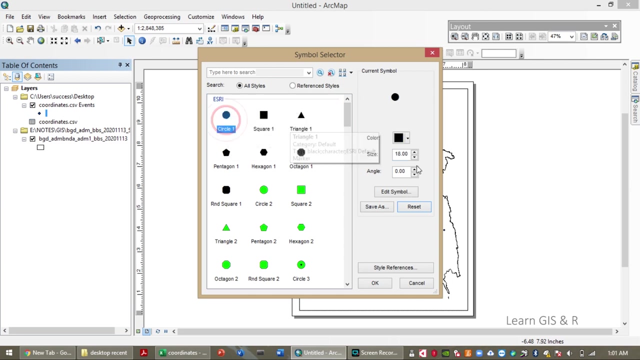 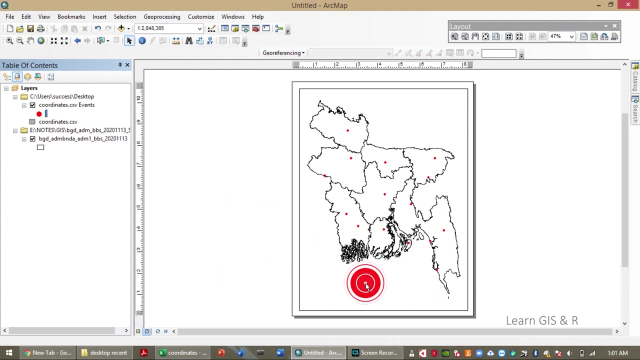 been imported. Now I'm going to display the coordinates. X field should be longitude and Y field should be latitude. Now the data points have been imported. here You can change the shapes of the points. I've just selected the round shape and selected red as the color. 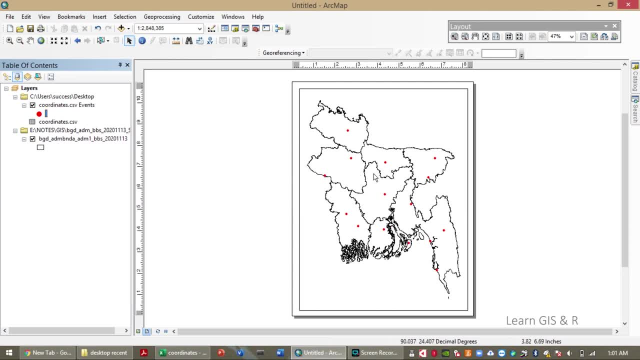 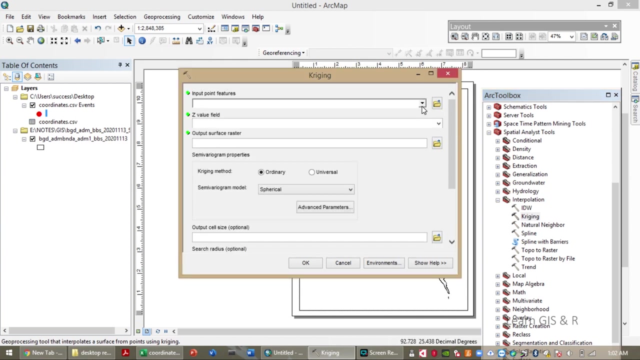 I'm going to leave it here. Open the arc toolbox. It may take some time to open. Open the spatial analysis tools and you have to go. interpolation techniques: There are multiple numbers interpolation techniques like IDW, create nearest neighbors line, etc. and there are some differences between the IDW and Kriging, which is 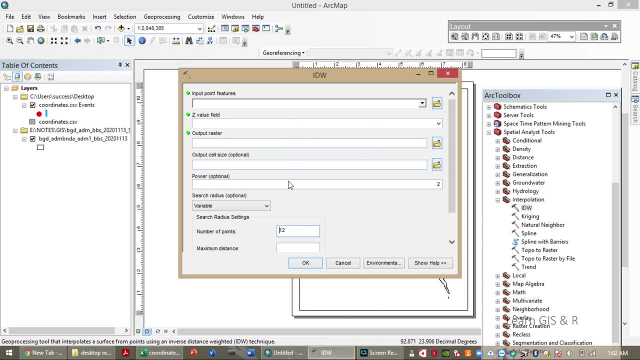 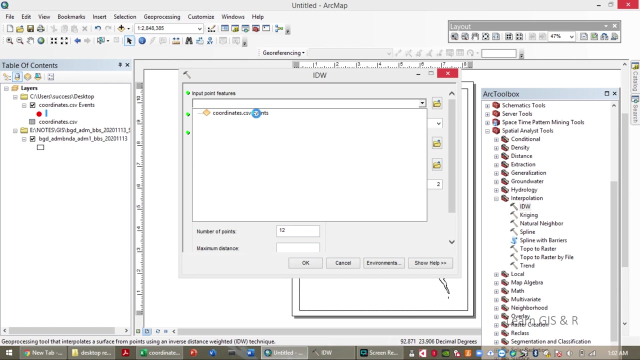 actually based on the topography or the geographic location. now, in this tutorial, I'm going to use IDW, which actually means inverse distance weighted function. now, if I select the CSV file as input point features, I don't know why, shame time. yes, you have to feel legit value, which you actually 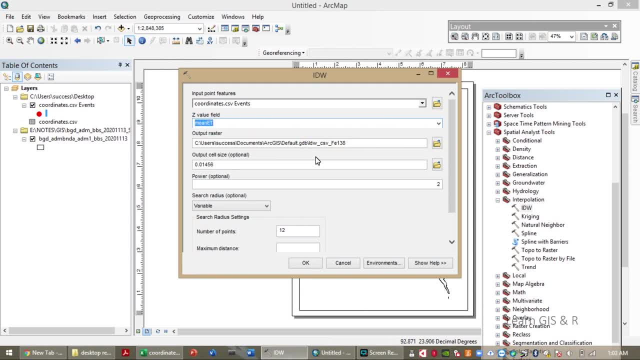 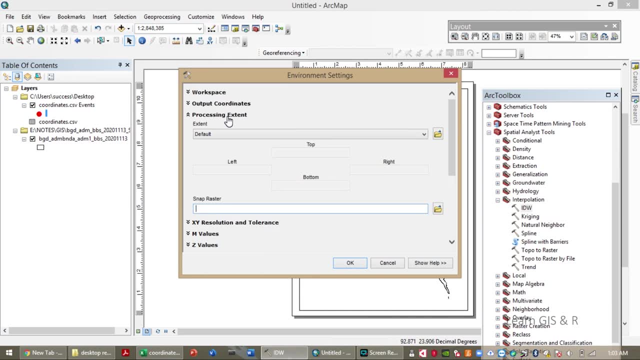 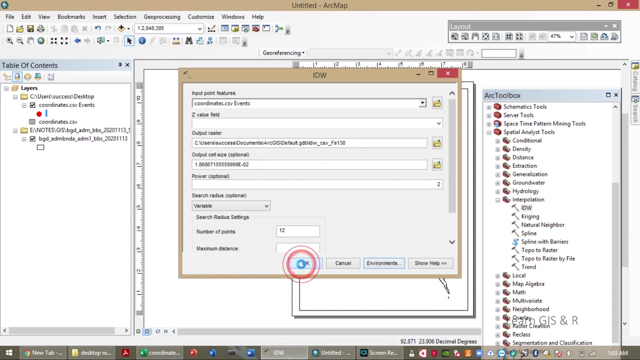 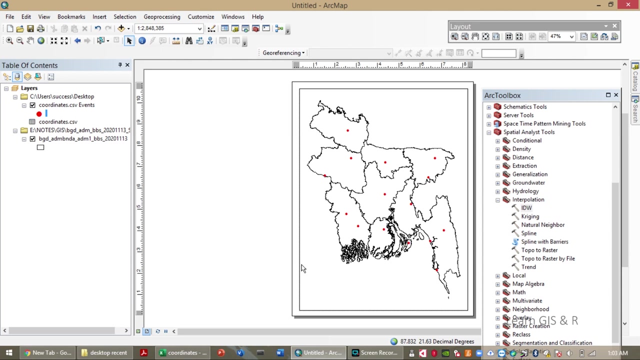 want to show in this in your map or don't feel new, actually want to show the distribution or processing extent should be your story area and you have to select the roster analysis and mask your shape file for the spatial distribution. okay, oh, I found the error. if your system show this problem, don't worry, there is a. 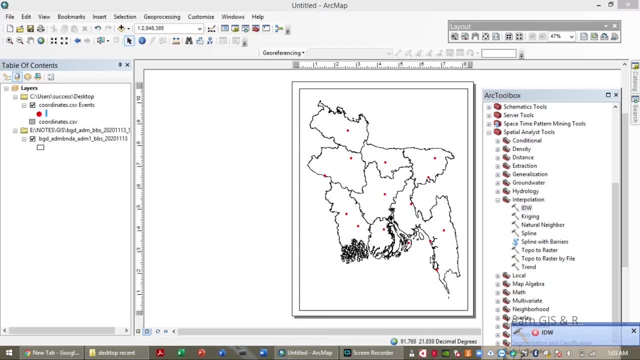 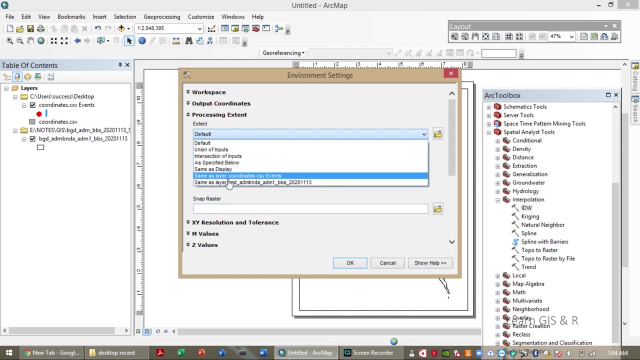 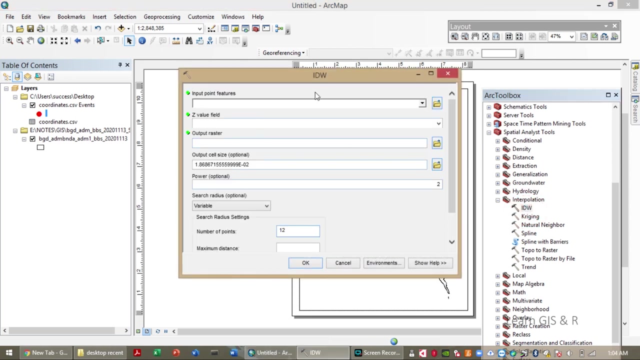 solution: exit your open CSV file and set your environment before going to conduct the analysis. now I'm selecting my environment before conducting my analysis and it can be a solution for this error. you okay, I think now it will be solved. IDW actually determines so values using. 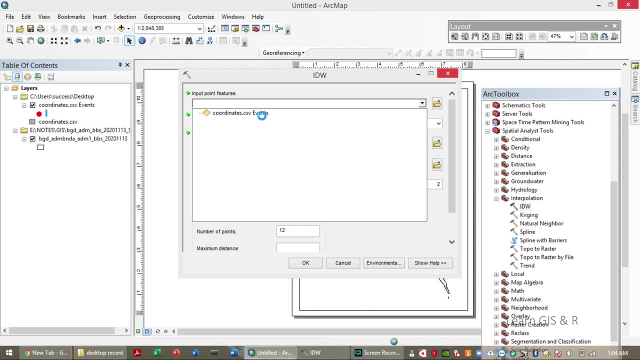 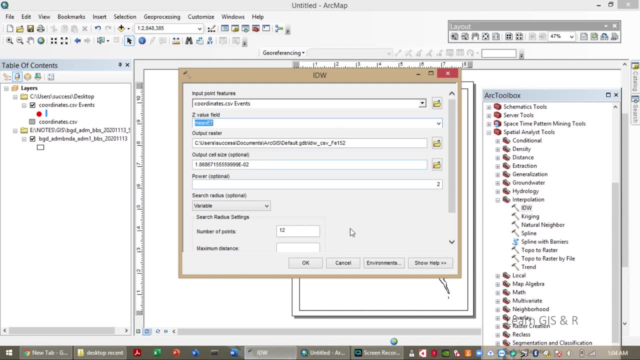 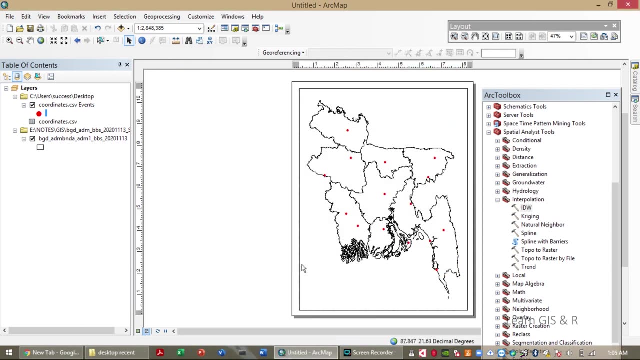 a linearly weighted combination of a set of simple points. the weight is a function of the inverse distance between them. the surface should be that of a locationally dependent variable. the messeited are closest to the unrok. Commissioner, it has the most influence. I mean that have the most. 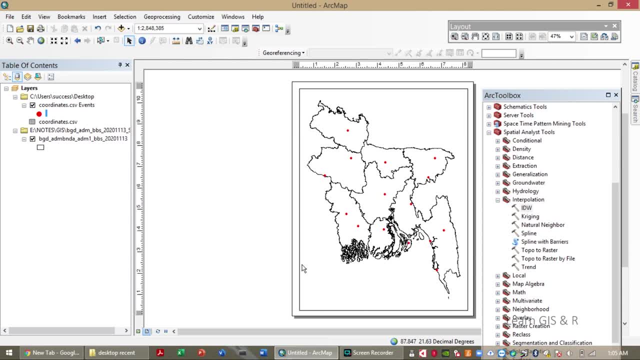 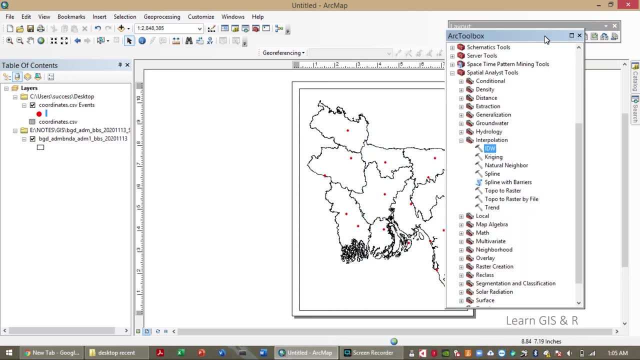 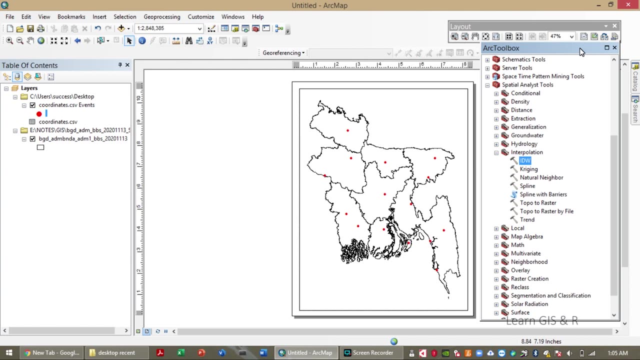 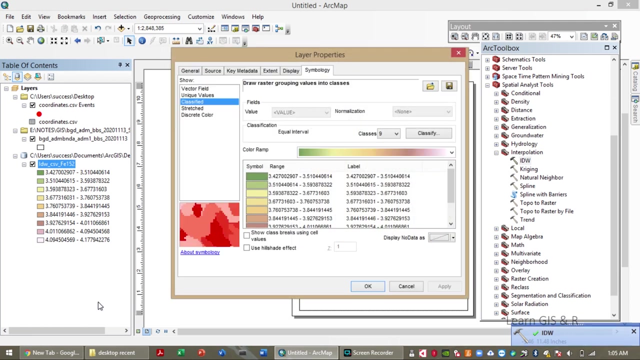 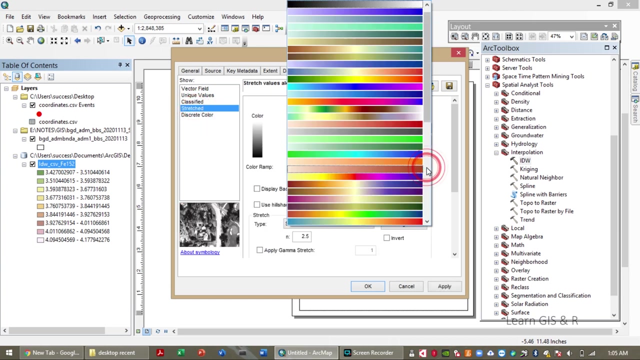 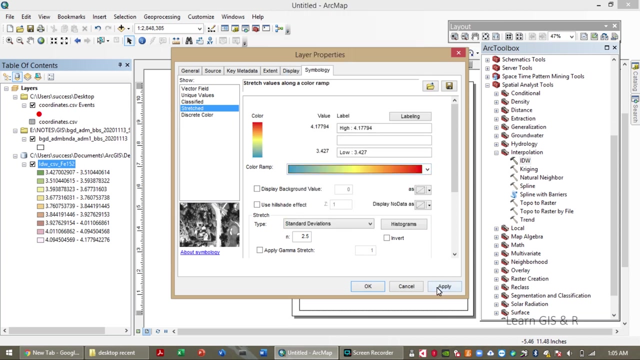 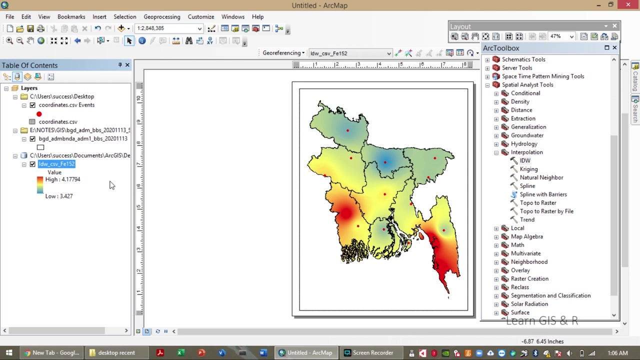 influence values. kid analysis is running background so we have to wait to show the results. yes, I find I found the initial results from the IDW method. you can use the stressed or classified. I'm going to use the stress values from this analysis. okay, the spatial analysis have been done. 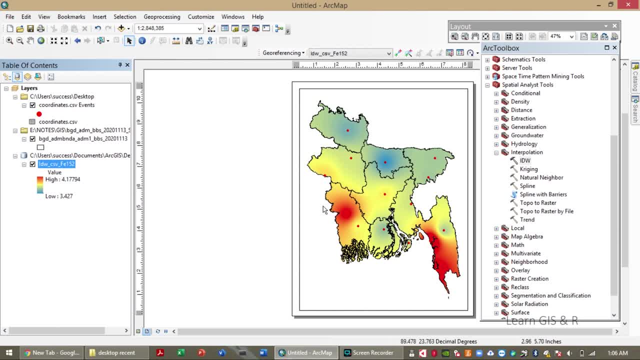 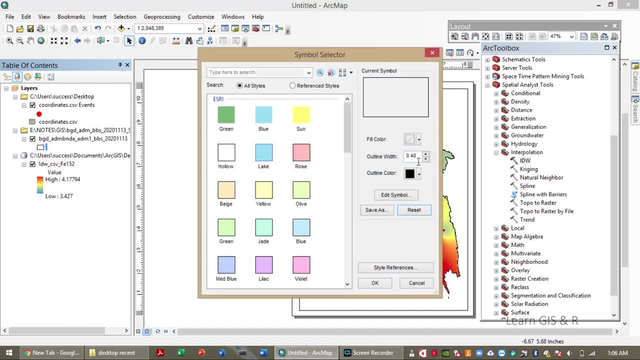 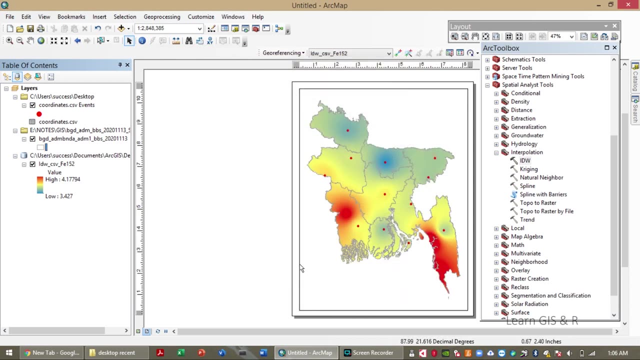 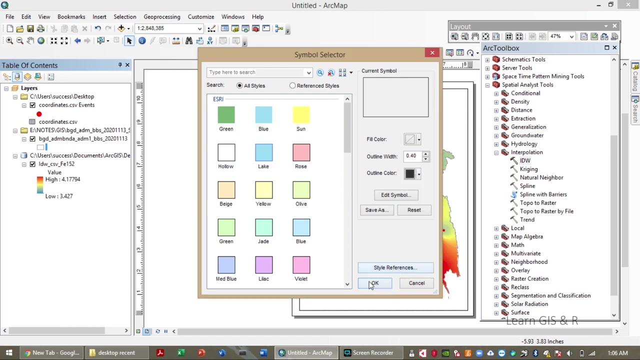 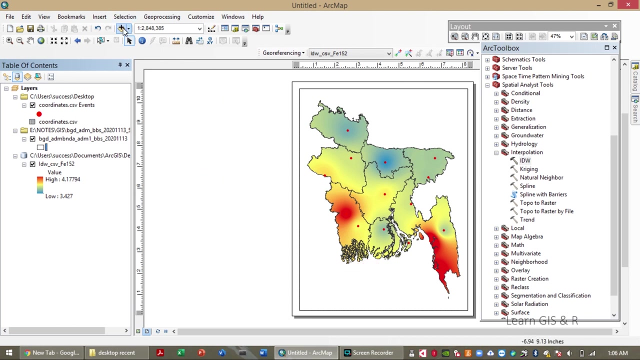 I think I need to change the shapefile because in next I want to show the contour lines in this spatial analysis map. therefore, I need to change the shapefile. actually, I don't want lines in the maps, so I think I should use only the country shapefile. that would be a solution of 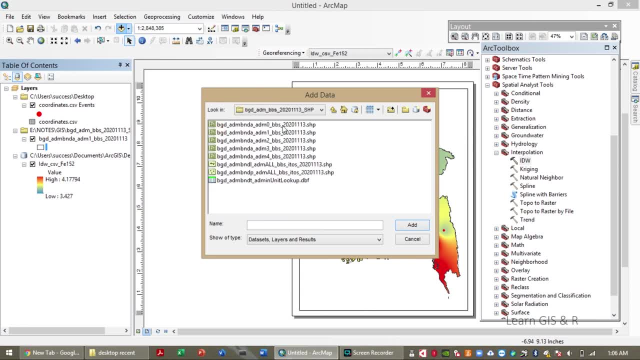 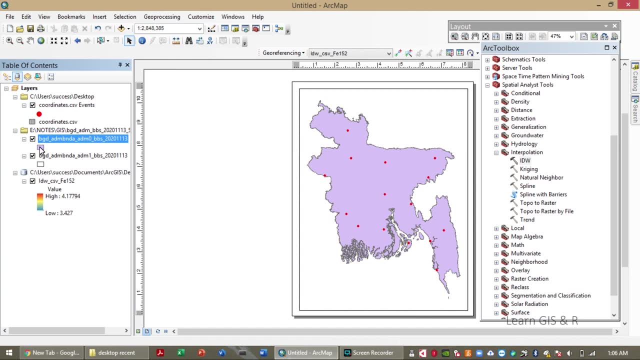 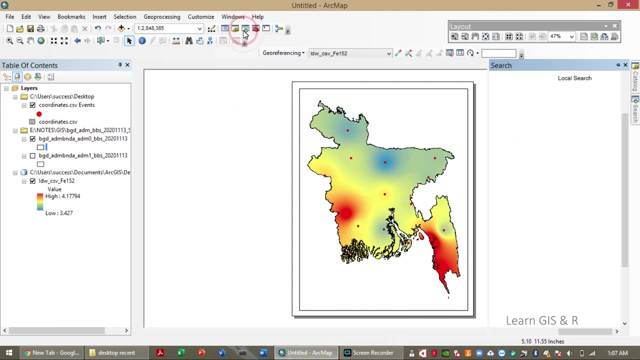 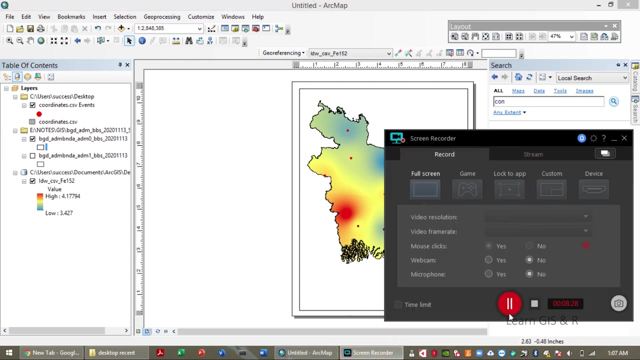 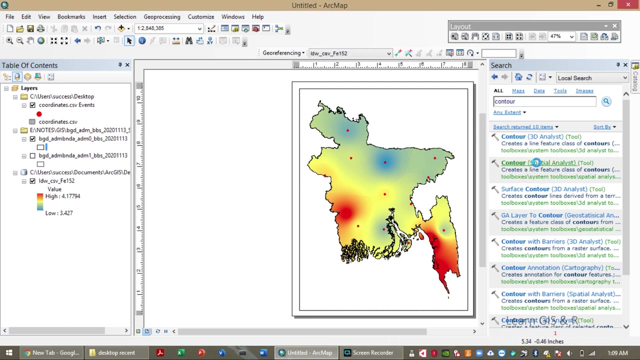 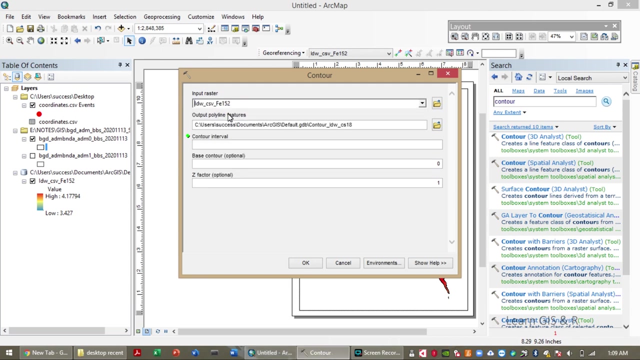 this. yes, I think this will be the solution. yeah, yeah, yeah, yeah, open the search toolbox and write contour in search box and open the contour from spatial analysis tool. yes, the contour interval actually depends on your values because, as i have the maximum value of 4.18, 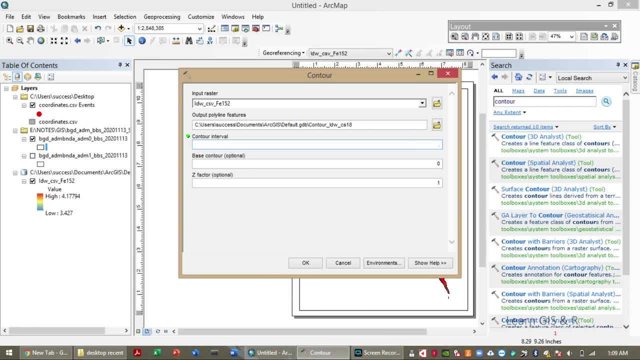 approximately, and the lowest value was 3.42. that's why i think 0.2 will be the appropriate value for this analysis, or it depends on your criteria. okay, 0.2 would be the perfect for me. the content line actually shows which areas have the similar values. 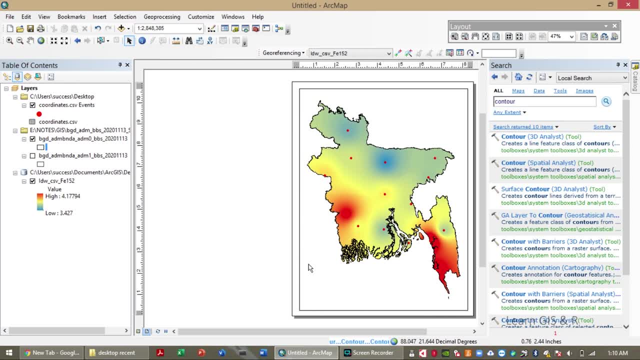 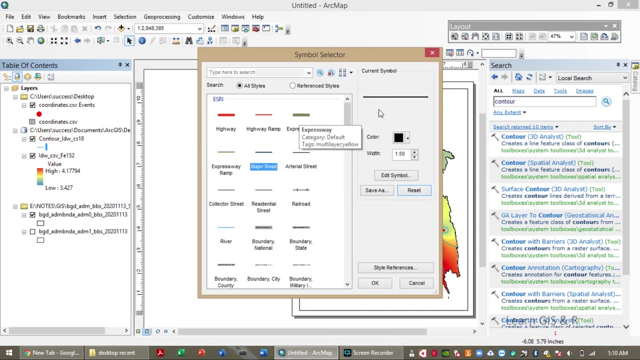 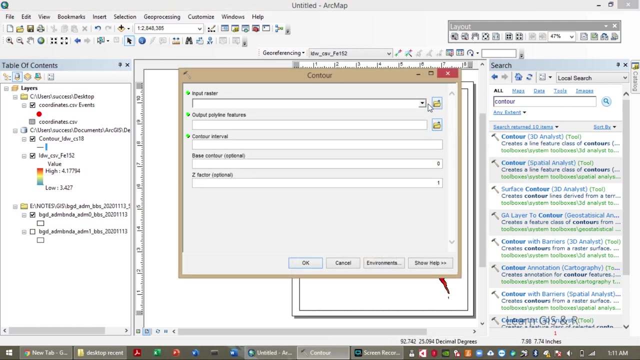 and it clusters. it clusters the areas from the shapefile with the similar values. i'm changing the color of the counters. okay, now i'm going to show you another counter with an interval of 0.1. it will show you more classes than before, so i think 0.2 would be the perfect interval for me. 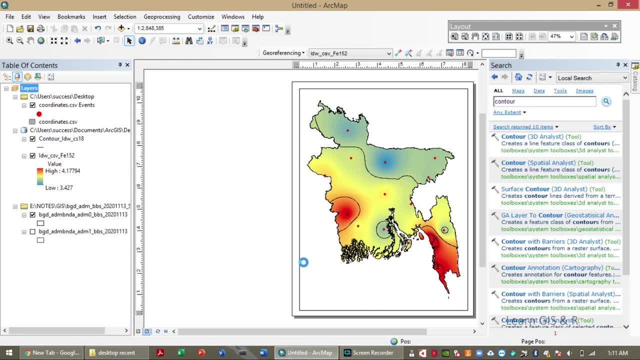 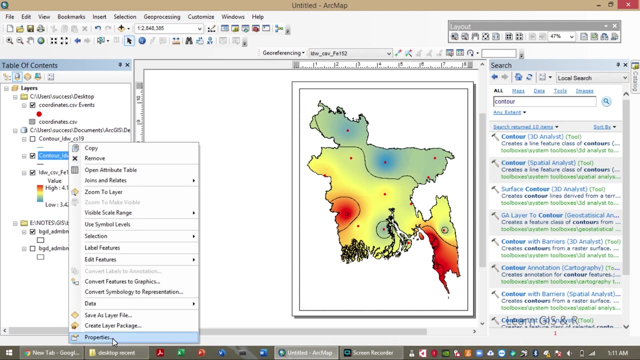 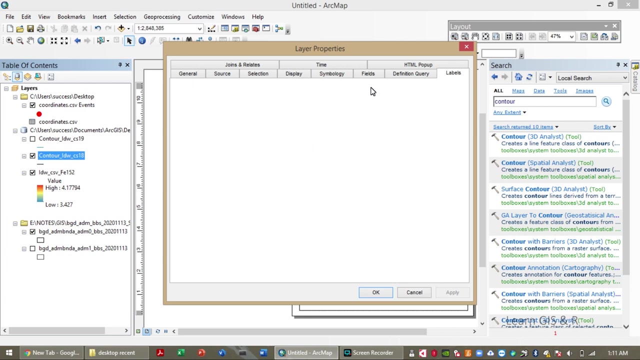 so i think 0.2 would be the perfect interval for me. i think it's going to keep. by the way, i think 0.2 will be very grounded level. if i have this set of values in my mind, it will keep away from my heart. 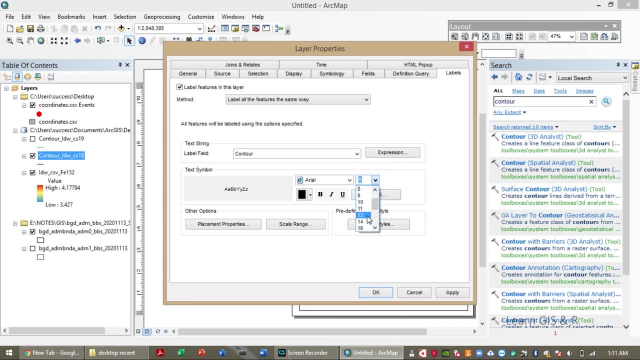 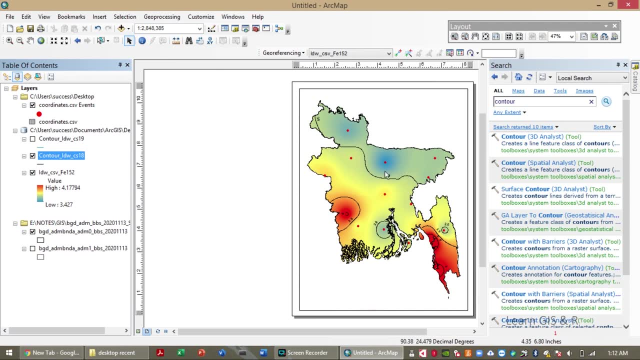 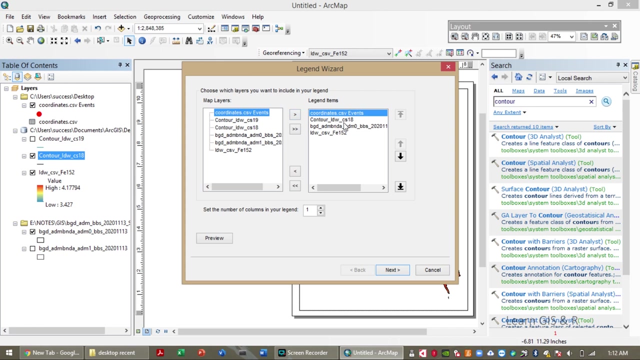 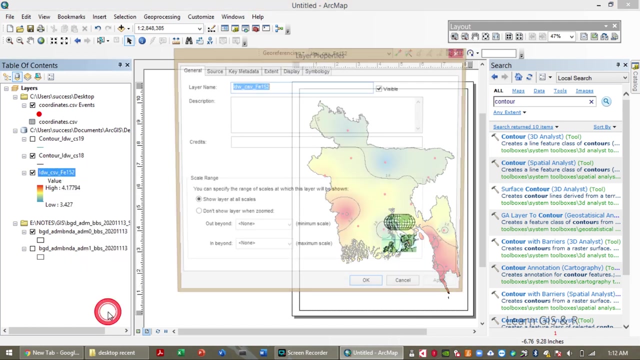 now i'm going to show you a three point-starх. okay, now the contour lines is showing the numbers or showing the values of evapotranspiration for my desired location. now I'm doing the typical map properties, including legend, inputting the coordinates, inputting the scale bar or the- not there right now, which is one of. 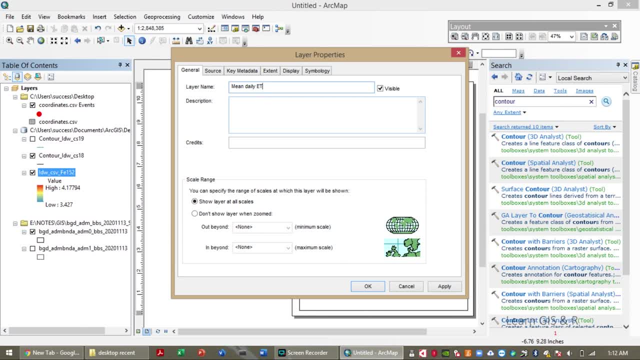 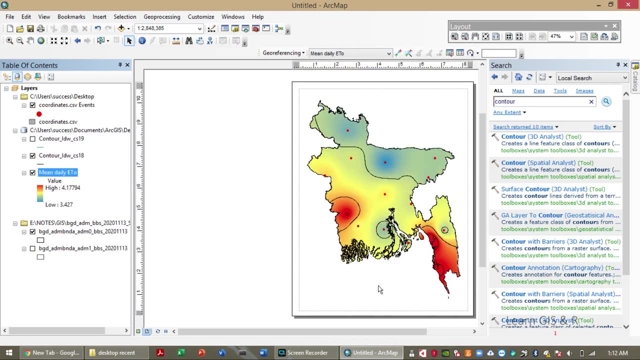 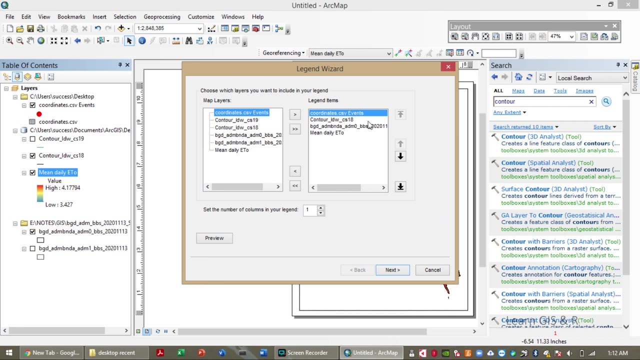 the most important criteria for map design. so follow the video for creating the distribution map. you can use this type of map for any analysis, or if you want to use, or if you want to. you can use this type of map for any analysis, or if you want to use, or if you want to. 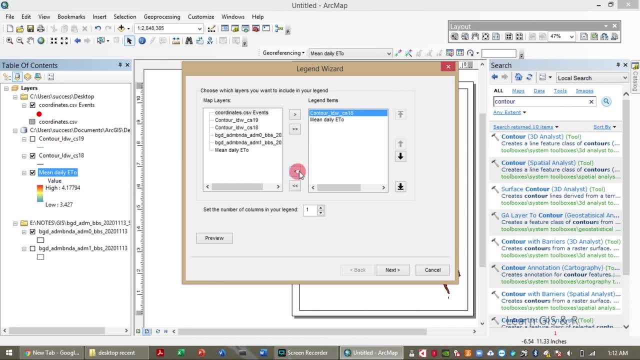 explain the noise levels, pollution or any other chemical characteristics for your desired location. I think this video is for you- is showing how to create a map of spatial distribution using IDW method. you can use the create, use the creaking and there are. there is there are some differences between IDW and 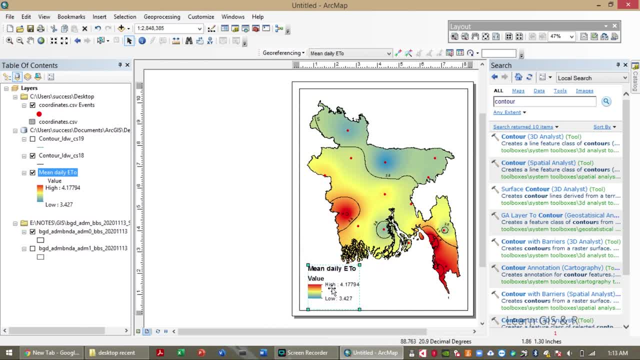 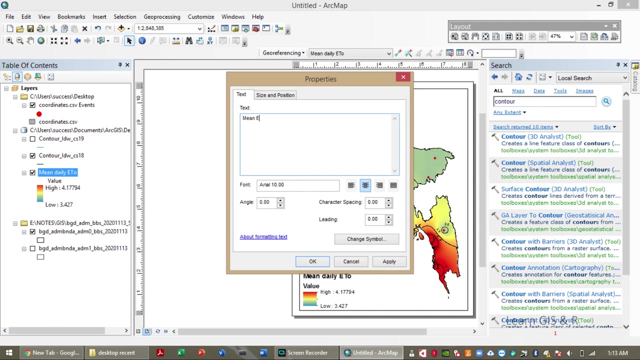 creaking and there are there are some differences between IDW and creaking method. some scientists actually recommends creaking, which is generally precise than IDW but triggers certain expertise and acquaintance with a topographic situation. core assumption of creaking is that spatial correlation within the 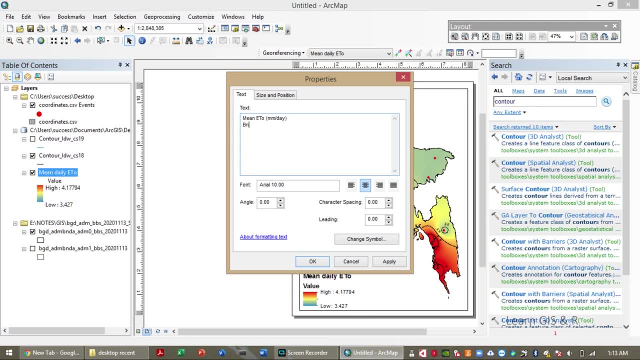 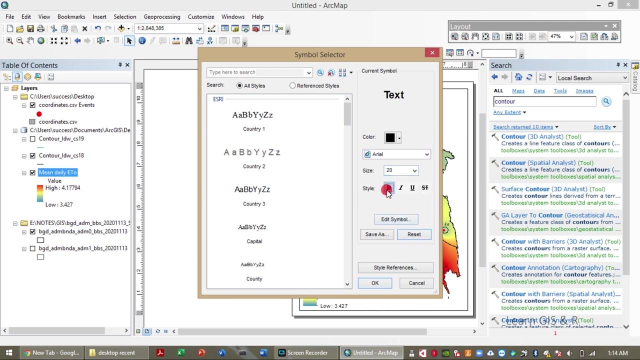 area is changing. use creaking if there is a spatially correlated distance or bias in the data, or you can use simply IDW method, because it is more simpler than any other interpolation technique. the IDW actually determines cell values using a linearly weighted combination of a set of sample points. 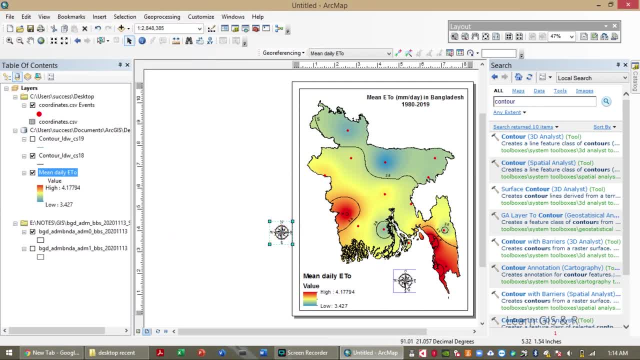 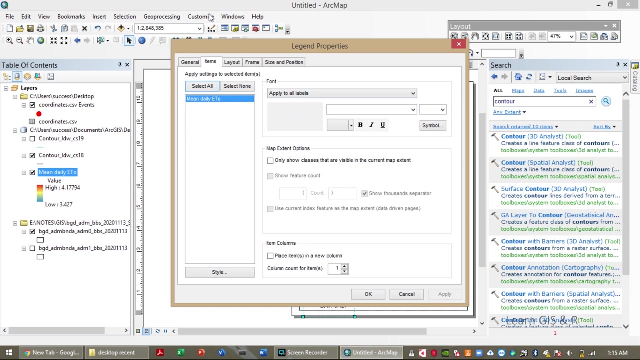 you can calculate it mean errors or RMSE of each method and compare them. I will explain my next video where you have to use the IDW and where you have to use the creaking or nearest neighbor method for interpolation technique, as IDW interpolation is one of the simplest and most popular interpolation. 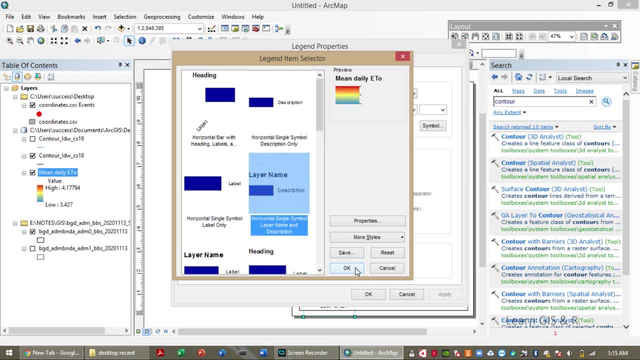 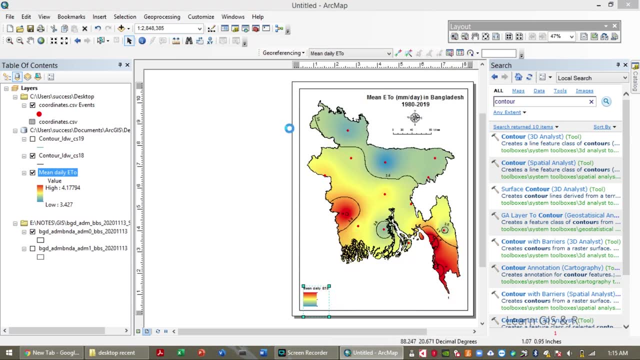 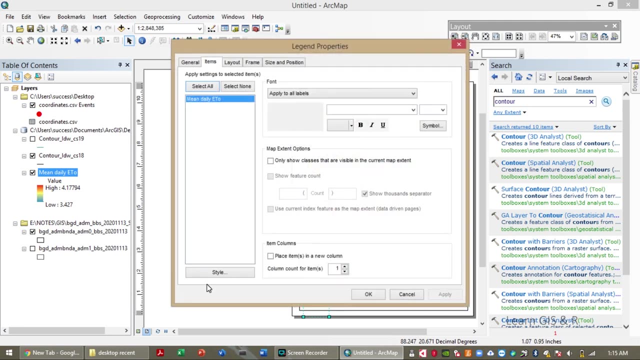 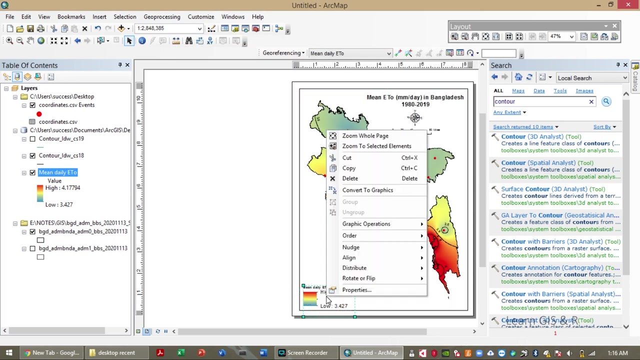 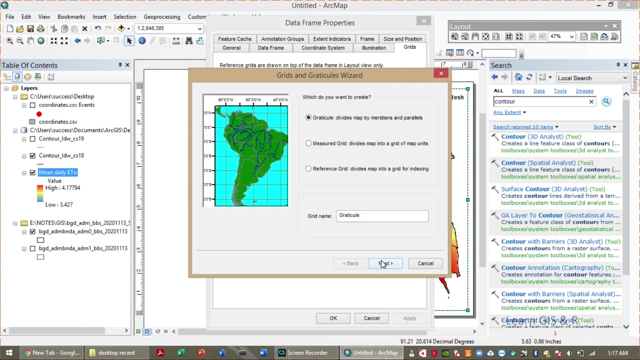 techniques for continuous variable modeling. I have used this method in this video. you the map has been created. the only thing I need to input is the coordinates of the map has been created. the only thing I need to input is the coordinates of the map and the coordinates of the map and the coordinates of the map and the coordinates of the map.